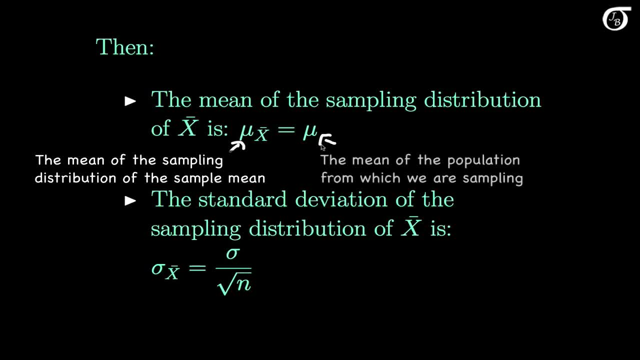 and that is equal to the mean of the population from which we are sampling. Or, in other words, the expectation of our random variable X bar is equal to mu, the mean of the population from which we are sampling. The standard deviation of the sampling distribution of X bar. 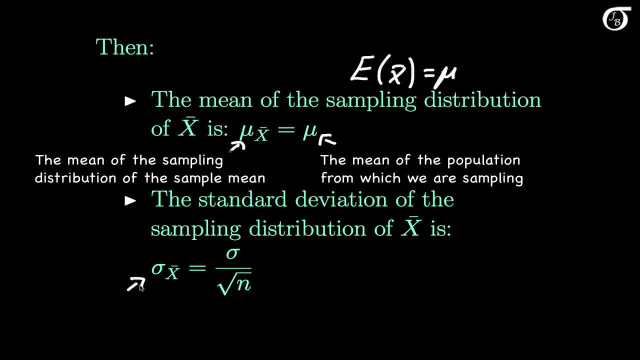 which will represent by sigma, with a subscript of X bar, is equal to the standard deviation of the population from which we are sampling divided by the square root of the sample size, And the standard deviation is just the square root of the variance, and so the variance of X bar is equal to that quantity squared. 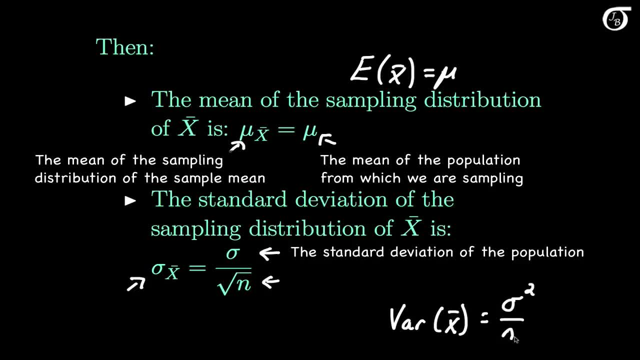 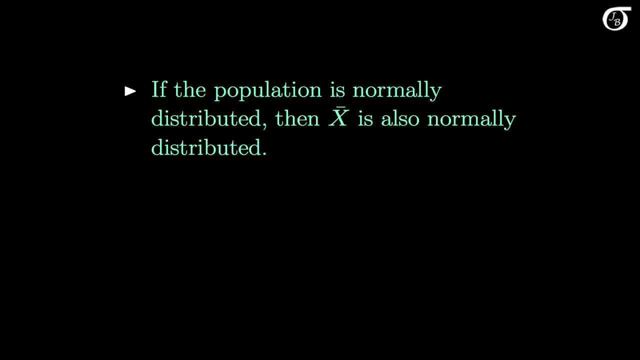 or in other words sigma squared over n. If the population from which we are sampling is normally distributed, then X bar is also normally distributed. And so, in summary, if we're sampling n observations from a normally distributed population, X bar is distributed normally, with a mean mu and a variance of sigma squared over n. 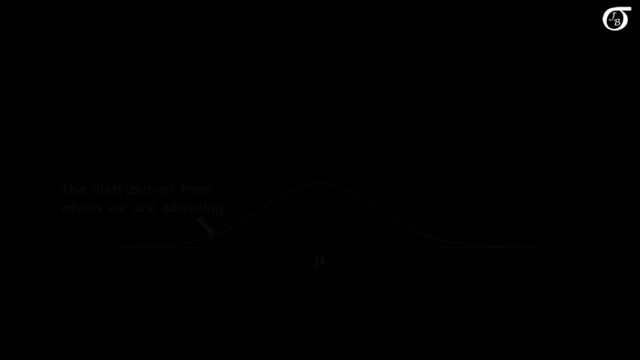 Let's see what that looks like. Suppose we're sampling from this distribution, which is a normal distribution with a mean of mu and a standard deviation of sigma. This distribution given in red is the sampling distribution of the sample mean X bar for a sample size of 2.. 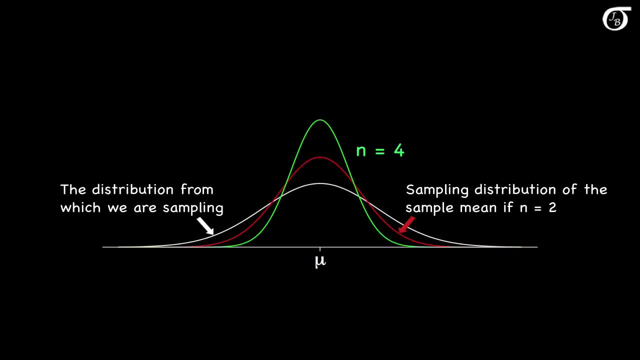 The distribution in green is the sampling distribution of X bar for a sample size of 4,. and the distribution in orange is the sampling distribution of X bar for a sample size of 8.. In all of these situations, the mean of the sampling distribution 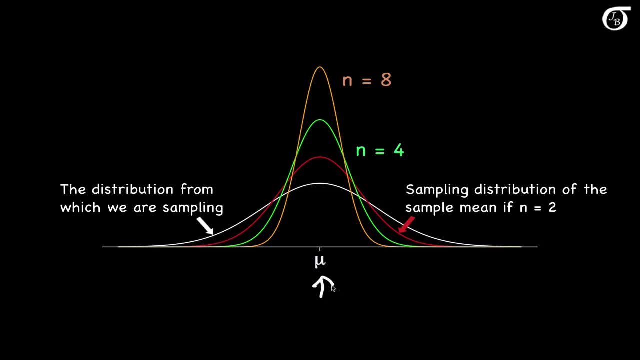 is always equal to the mean of the population from which we are sampling, But the standard deviation is smaller Here. the standard deviation of the population from which we are sampling, represented by the white curve, is sigma When the sample size is 2,. 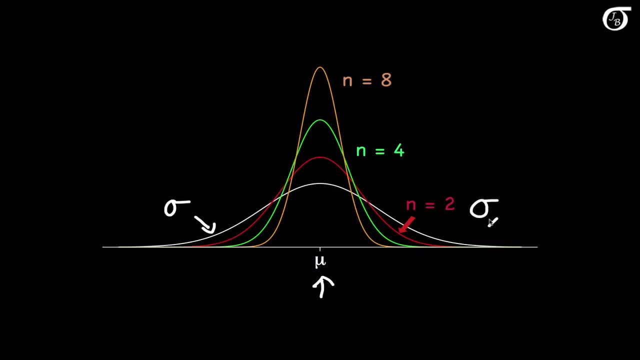 the standard deviation of the sampling distribution of X bar, which we represent by sigma. X bar is equal to sigma over the square root of 2.. And when the sample size is 4, the sampling distribution of X bar has a standard deviation of sigma over the square root of 4.. 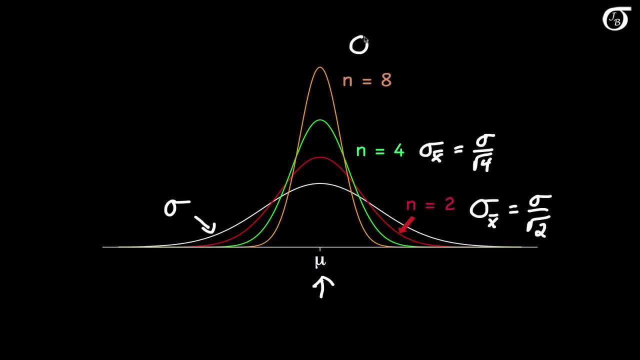 And when the sample size is 8,, like in the orange curve, the standard deviation of the sampling distribution of X bar is equal to sigma over the square root of 8.. So the standard deviation of the sampling distribution of X bar decreases as the sample size increases. 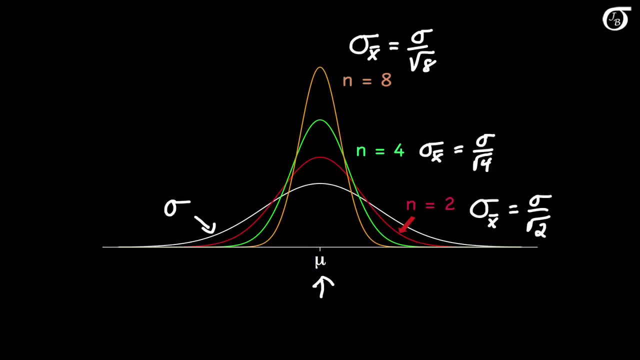 But it decreases by a factor of the square root of the sample size. So if we wanted to cut the standard deviation of the sampling distribution in half, we would need to quadruple the sample size, A main reason we like large sample sizes in statistics. 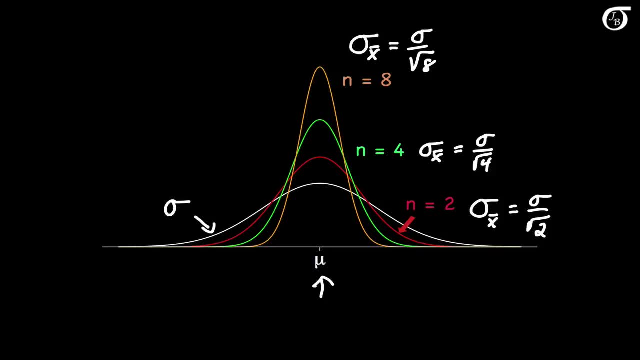 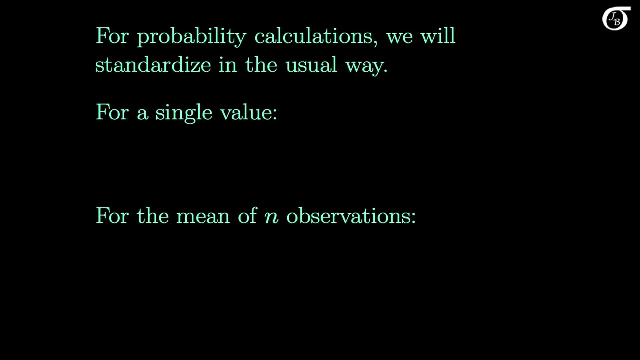 is that for a larger sample size, the distribution of a statistic is going to be more tightly grouped around the parameter it estimates, And so we're going to be able to estimate that parameter with greater precision In probability calculations. we will standardize in the usual way. 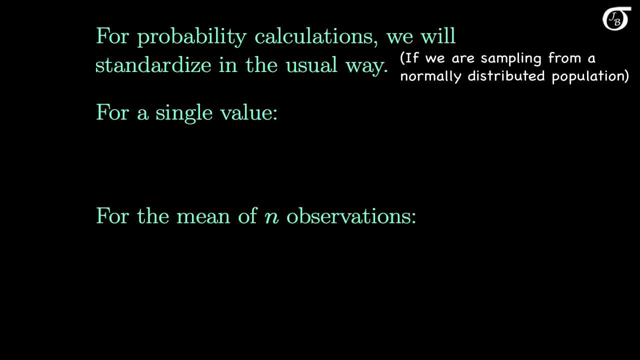 If we are sampling a single value from a normally distributed population, then that single value, X say, has a normal distribution with a mean of mu and a variance of sigma squared. To standardize, we subtract the mean and divide by the standard deviation. 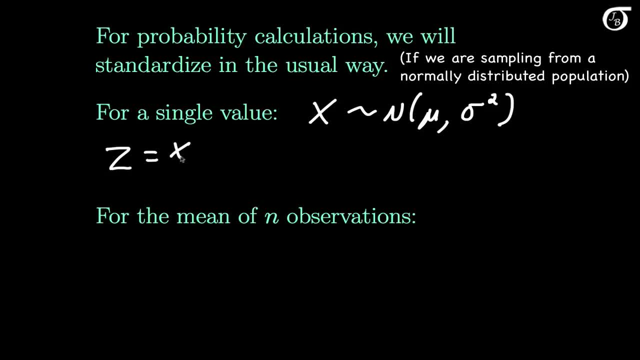 So if we let the random variable Z equal X minus its mean of mu and divide by its standard deviation of sigma, then Z has the standard normal distribution For probability calculations involving the mean of n observations. X-bar is distributed normally with a mean of mu and a variance of sigma squared over n. 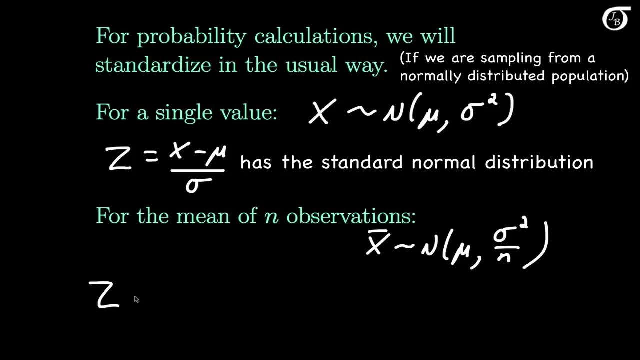 And so to standardize here, we're going to let the random variable Z equal X-bar minus its mean, which is simply mu, and divide by the standard deviation of X-bar, which is sigma over the square root of n. And if we subtract the mean of mu and divide by the standard deviation of X-bar, 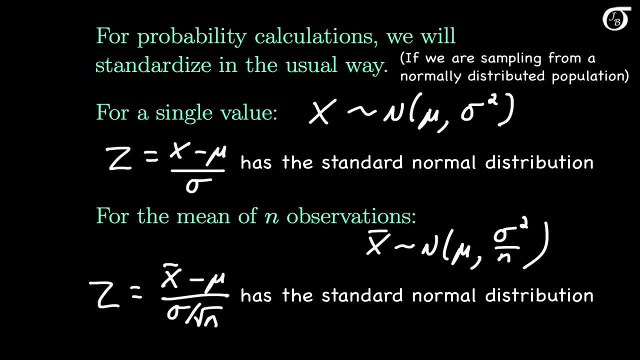 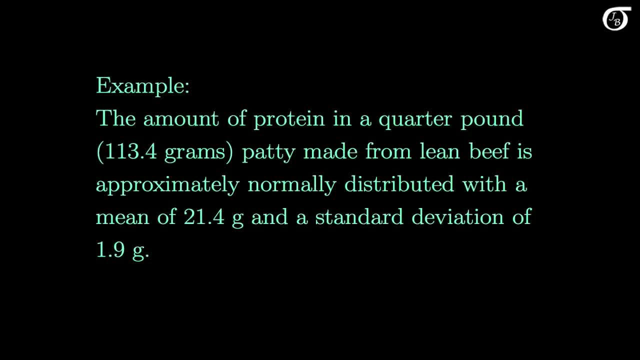 and if we do that, then the random variable Z is going to have the standard normal distribution. Let's look at an example of this type of probability calculation: The amount of protein in a quarter pound patty, or about 113 grams of lean beef. 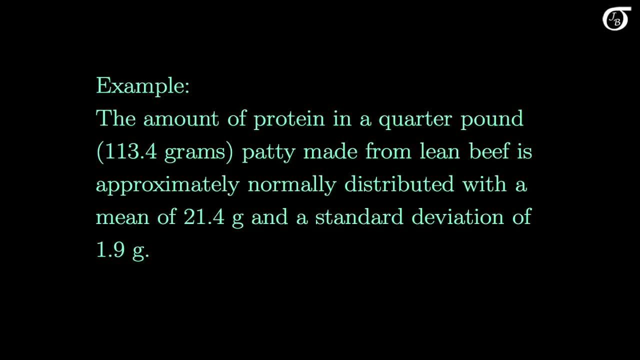 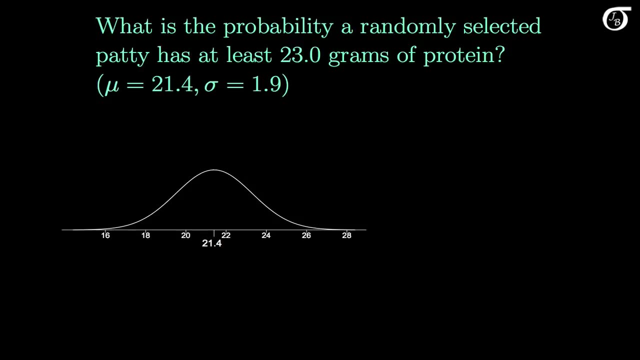 is approximately normally distributed, with a mean of 21.4 grams and a standard deviation of 1.9 grams. This is based on information from the USDA nutrient database. Suppose we want to know the probability that a single randomly selected patty has at least 23.0 grams of protein. 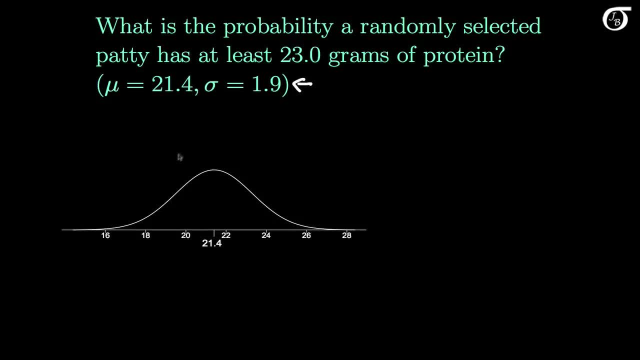 Here again are the mean and standard deviation for the population, and I've plotted in the distribution of the amount of protein in a single burger here. And if we let the random variable X represent the amount of protein in a randomly selected burger, then here we want to know the probability that the random variable X takes on a value that's at least 23.0. 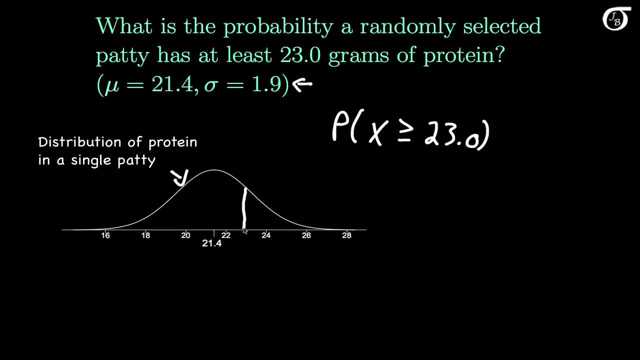 And that is simply the area of protein in a single burger. That is the area to the right of 23.0 under this distribution, this area right here To find that we can standardize by subtracting the mean and dividing by the standard deviation. 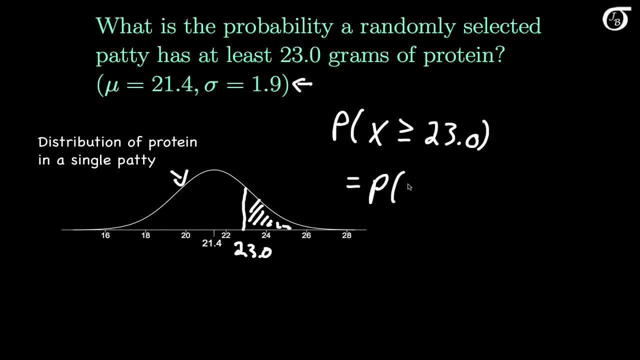 And this is equal to the probability that the random variable Z, where Z has a standard normal distribution, takes on a value that's bigger than or equal to 23.0 minus the mean of 21.4 divided by the standard deviation of 23.0.. 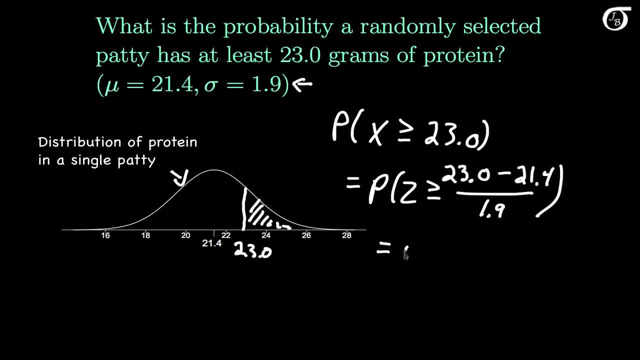 And that's simply equal to the probability that the random variable Z takes on a value that's bigger than or equal to 0.842.. And we draw out our standard normal curve: 0 in the middle out here somewhere is 0.842,. 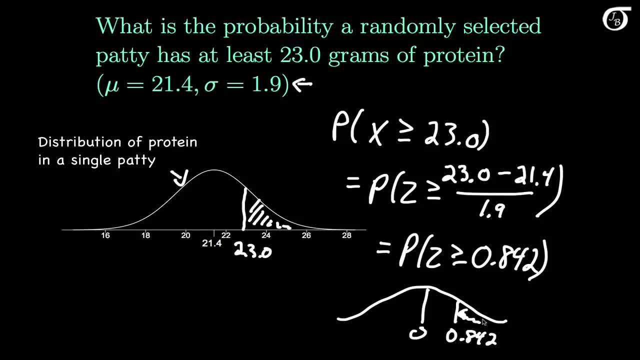 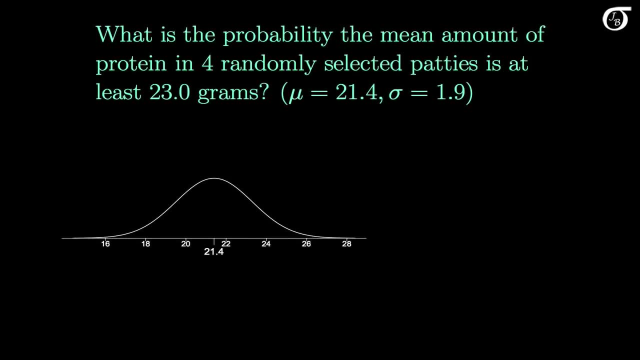 and we need this area here. If we go to software or a standard, normal table, we can find that to three decimal places, 0.200.. So that's the probability we're looking for. That last question involved the amount of protein in a single patty. 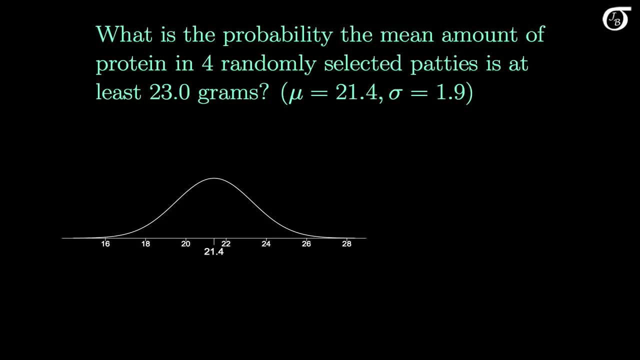 And here the question changes a little bit. What is the probability? the mean amount of protein in four randomly selected patties is at least 23 grams. Here again in white, is the distribution of protein in a single patty. But in this question we're interested in the probability based on the mean amount of protein in four patties. 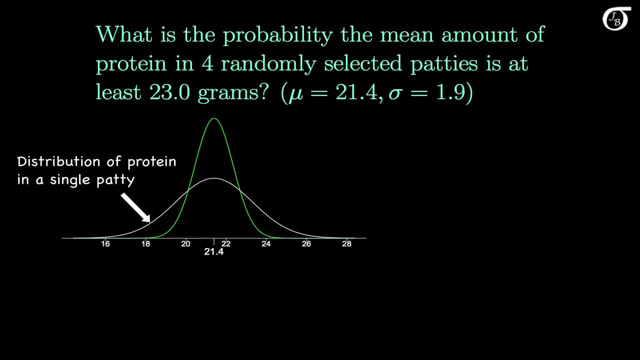 And I'm going to draw in this curve in green, which is the sampling distribution of the sample mean. in this scenario This sampling distribution has the same mean as the original population of 21.4, but the standard deviation of this sampling distribution in green. 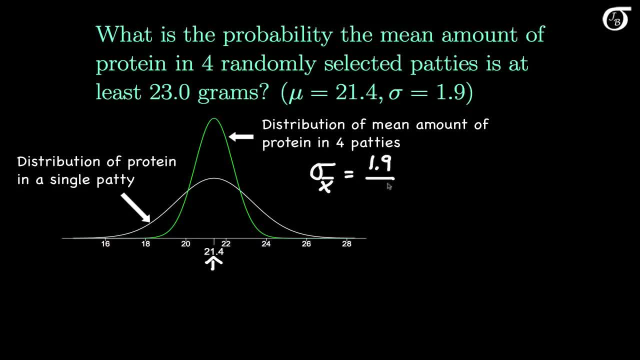 is sigma of 1.9 over the square root of n, which is the square root of 4.. And in this question we need to find the probability that the random variable X bar takes on a value that's bigger than or equal to 23.0.. 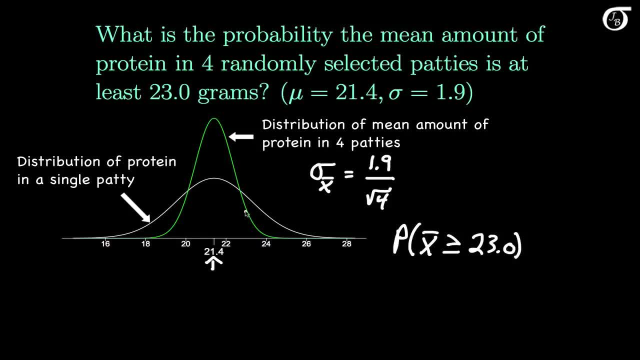 And that is going to be the area to the right of 23.0 under the green curve, under the sampling distribution of X bar, That area right there, And to find that probability we can again standardize. But we have to remember that when we're talking about the mean of n observations: 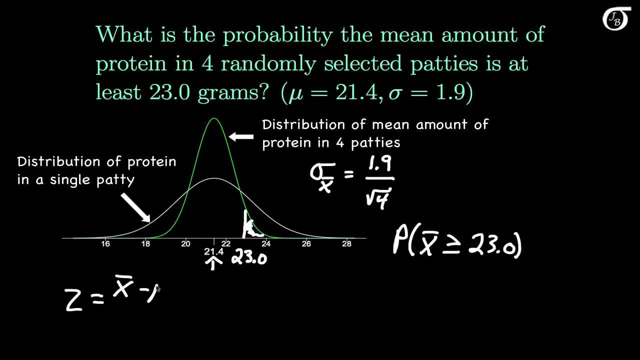 to standardize, we're going to let z equal X bar minus mu over sigma divided by n. So here this probability we're interested in, we're going to turn this into the probability that z is bigger than or equal to 23.0 minus 21.4. 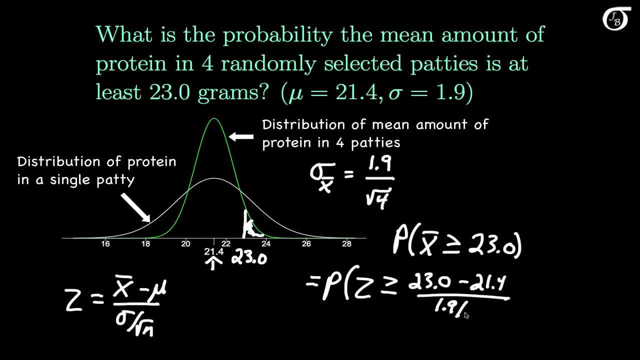 all over 1.9 divided by the square root of 4.. And this works out to the probability that z takes on a value that's bigger than or equal to 1.684.. And if we go to software or a standard, normal table, 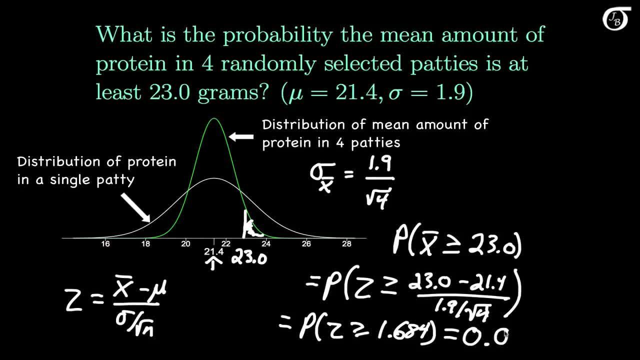 we can find that that probability to three decimal places is 0.046.. Here the distribution of the sample mean was approximately normal because we were sampling from an approximately normally distributed population. But there is a very important concept in statistics that helps us calculate probabilities involving the sample mean. 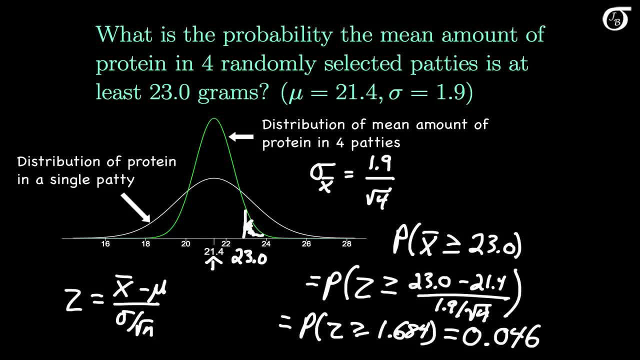 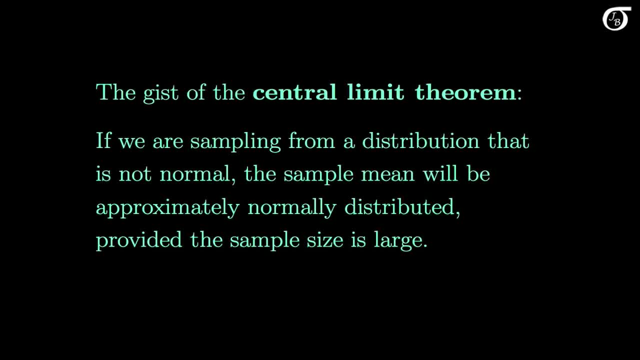 when we are sampling from distributions that are not normal. And let's take a quick look at that. The gist of the central limit theorem is that if we are sampling from a distribution that is not normal, the sample mean will still be approximately normal. 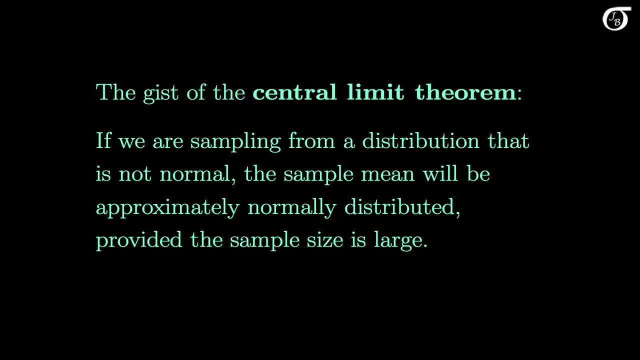 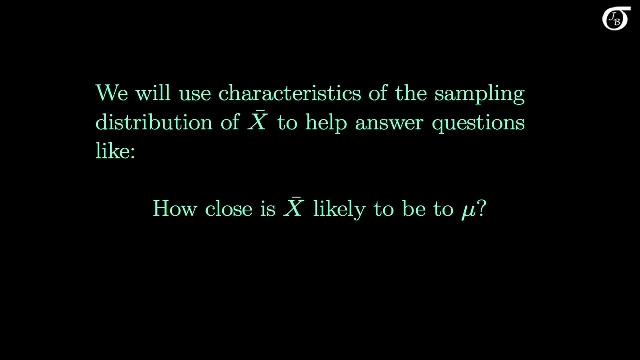 provided we have a large sample size. The central limit theorem is an extremely important concept in statistics and I'm just introducing it very briefly here, but I have another video that goes into it in greater detail. Why do we care about the sampling distribution of the sample mean?